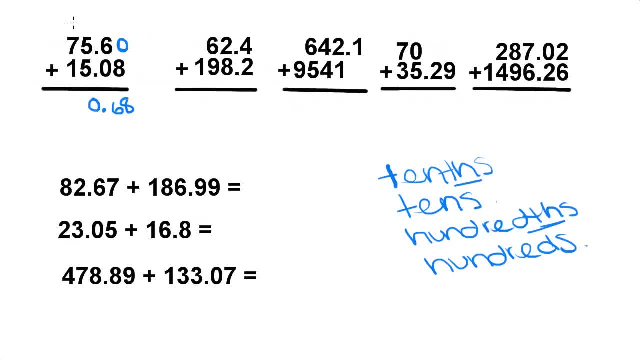 Five and five is ten. Put the zero there as a placeholder, Carry over the one. Seven, eight, nine And there's our product. So over here we do the same exact thing. Four and two is six. Bring down the decimal point. 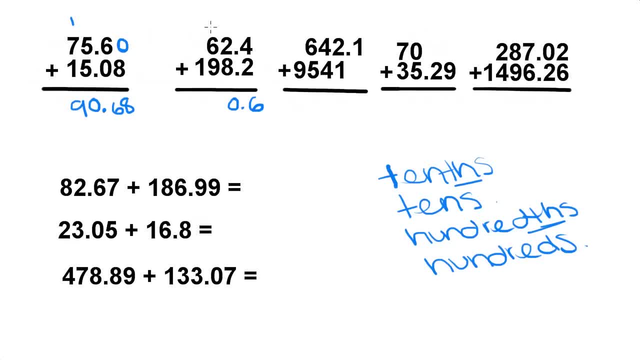 Eight and two is ten. Placement holder. Carry over the one. Nine and one is ten plus six is sixteen. Carry over the one. Bring down the six And one and one is two. It's a different color And over here. don't let this confuse. you Just put an imaginary decimal point right there and an imaginary zero as a placeholder. 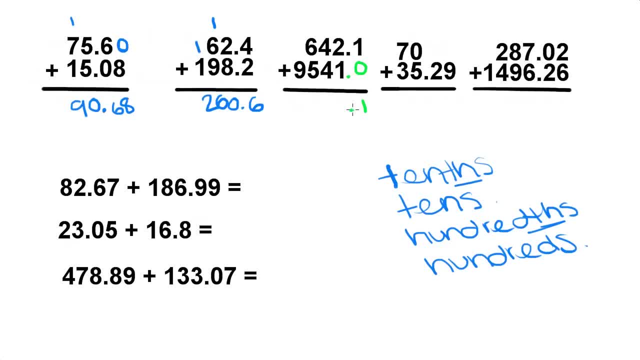 We have zero and one is one. Bring down the decimal point. We have two and one is three, Four and four is eight, Six and five is eleven. Put the one over there. Bring down the one right there And ten Same deal over here. Don't let this confuse you. 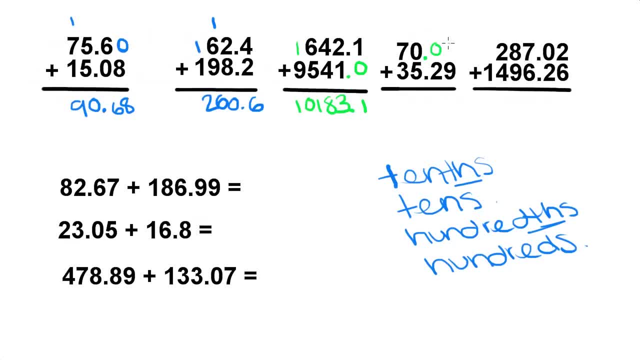 Put an imaginary little decimal point right there And two zeros. In actuality, there can be an infinite amount of zeros. So you can keep on going from so on and so on. So zero and nine is nine, Zero and two is two. 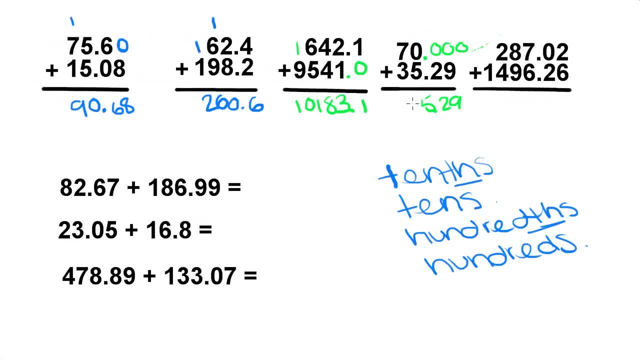 Bring down the decimal point Zero and five is five, Seven and three is ten. In this example, two and six is eight Zero and two is two. Bring down the decimal point Six and seven is thirteen. Carry over the one. 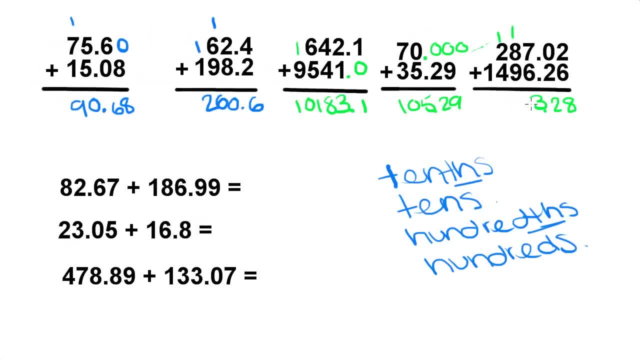 Nine and one is ten Plus eight is eighteen. Carry over the one, Bring down the eight. Four and two is six Plus one is seven And bring down the one And over here. if you get good at placement holders, you just know that there's two placements behind the decimal point. 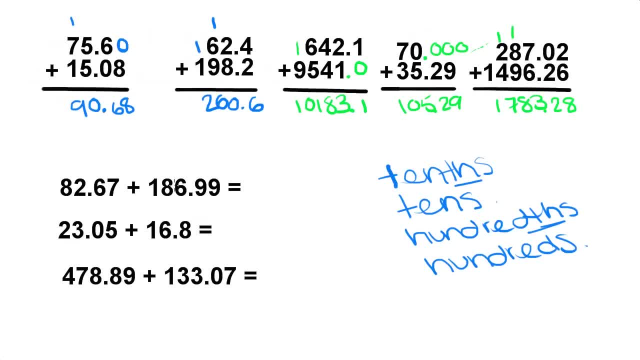 So you start with a seven and go two over, It's nine. Seven and nine is sixteen. You want to start way over here, Way to the right Carry over the one. You can put it wherever you want: On top of there, On top of there.